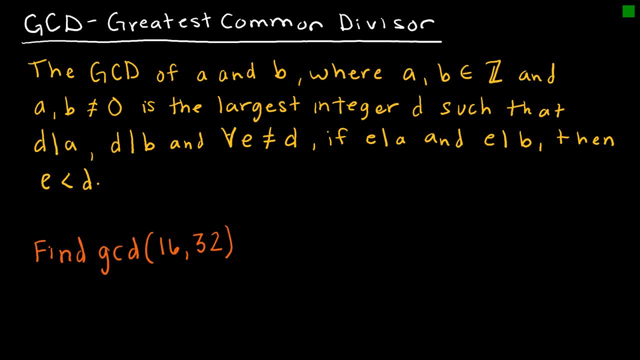 is the largest integer, such that D divides A and D divides B, And then essentially that is just saying that D is a divisor of both A and B. But then we throw in that for all E that is not equal to D if E also divides A and B. 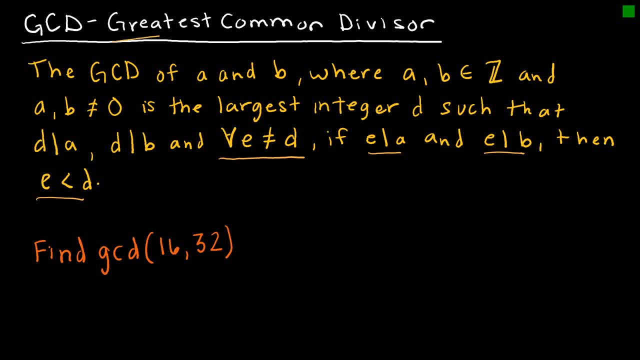 then E has to be less than D, And so that's what takes the greatest part of it. So it's the highest number, highest value, integer value, that divides both A and B. So pretty straightforward Again. I'm sure that we've all done these before. 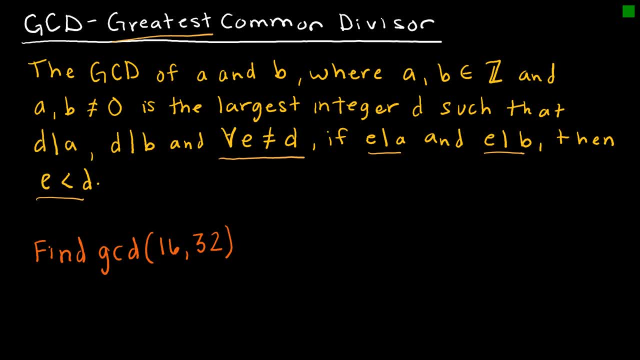 What I want to do is look at a few different ways that you can go about finding the GCD. So- and these are all again very elementary, So if I was looking at 16, I would say 16, the divisors are 1, because 1 goes into 16,. 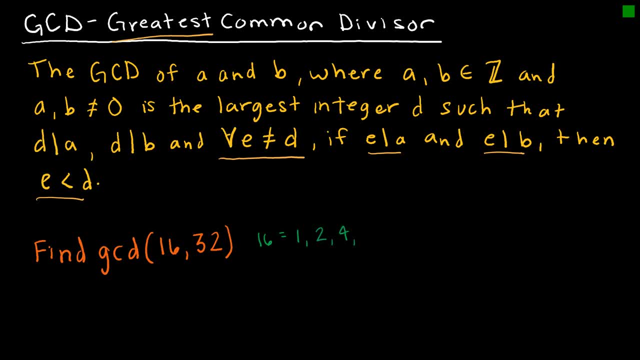 2,, 4 goes into 16,, 8 goes into 16, and 16 goes into 16.. And then I could do the same for 32.. So 1 and 2, and 4 and 8.. And again we're just looking for the one that that matches basically matches up and 16 and 32.. 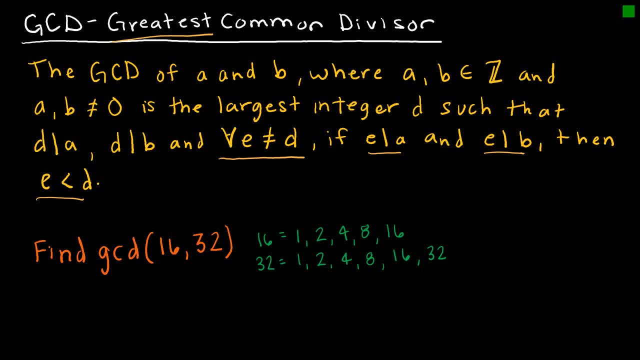 And so, again, all I'm looking for is what is the highest number that appears in both of those lists, and that number is 16.. So, again, I don't have to explain to you how to find a GCD. I'm sure you've done it several times. 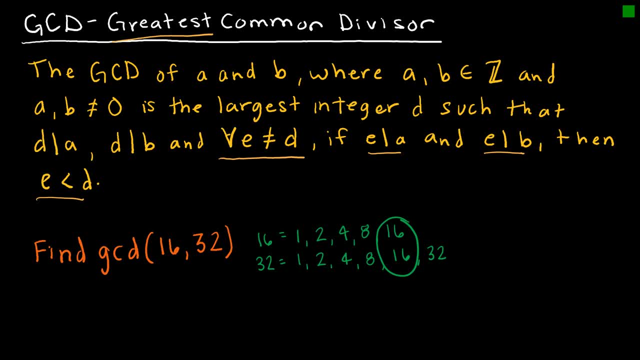 But now let's take a look at how I could do this using prime numbers, because obviously we're dealing with primes right now. So I could look at 16 and look at the prime factorization and the GCD or, I'm sorry, the prime factorization of 16, again, I could make a tree if I needed to. 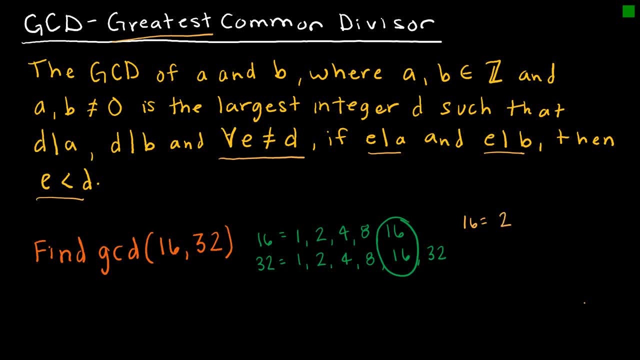 But really I'm just saying it's 2 times 2, times 2 times 2, or 2 to the fourth, And then, if I write 32, as the prime factorization, it's 2 to the fifth. And if I'm looking at the GCD, 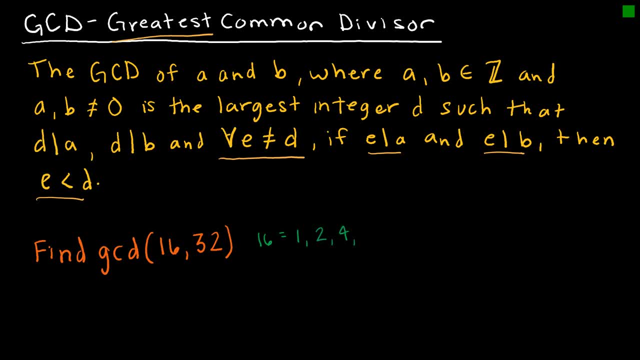 2,, 4 goes into 16,, 8 goes into 16, and 16 goes into 16.. And then I could do the same for 32.. So 1 and 2, and 4 and 8.. And again we're just looking for the one that that matches basically matches up and 16 and 32.. 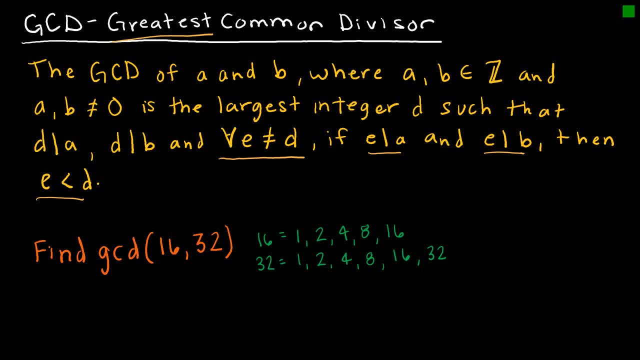 And so, again, all I'm looking for is what is the highest number that appears in both of those lists, and that number is 16.. So, again, I don't have to explain to you how to find a GCD. I'm sure you've done it several times. 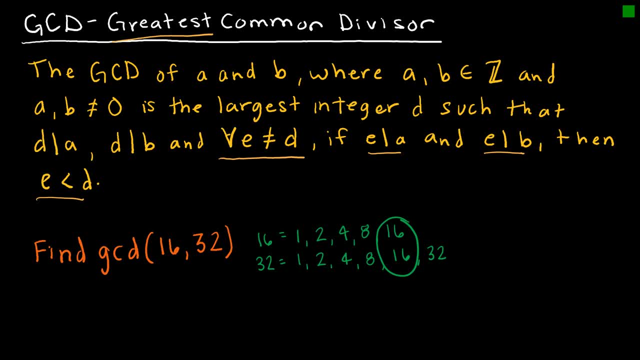 But now let's take a look at how I could do this using prime numbers, because obviously we're dealing with primes right now. So I could look at 16 and look at the prime factorization and the GCD or, I'm sorry, the prime factorization of 16, again, I could make a tree if I needed to. 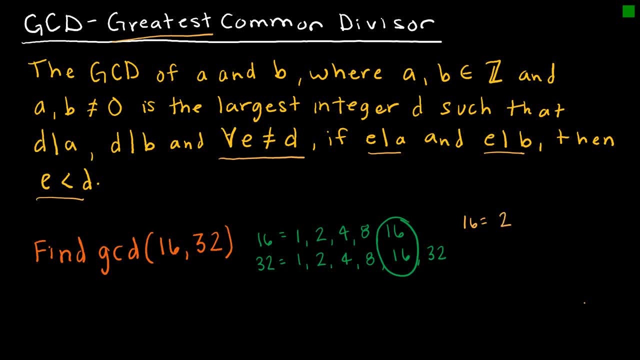 But really I'm just saying it's 2 times 2, times 2 times 2, or 2 to the fourth, And then, if I write 32, as the prime factorization, it's 2 to the fifth. And if I'm looking at the GCD, 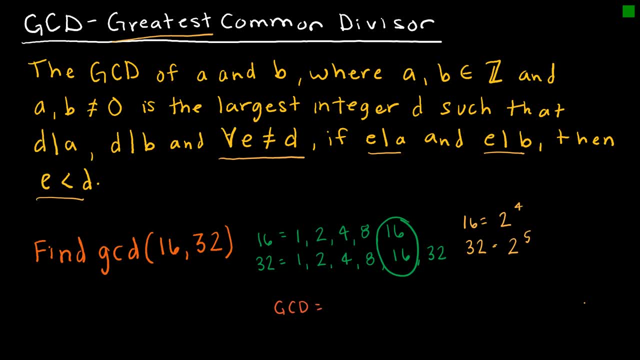 I'm looking at the most number of times that a prime occurs in common with one another. So here's 2 to the fourth, this is 2 to the fifth, So 2 to the fourth, and this is like 2 to the fourth times 2.. 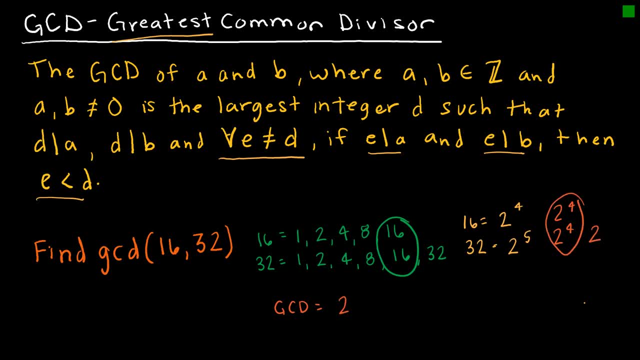 So 2 to the fourth is the greatest number of times that occurs in both, And so that is the greatest, And so that is the greatest common divisor, which is of course 16.. So the answer is 16, either way you look at it. 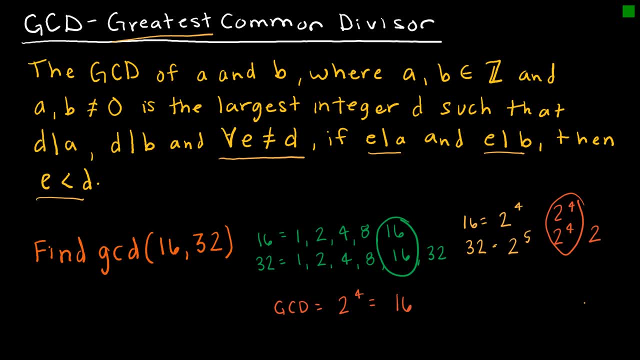 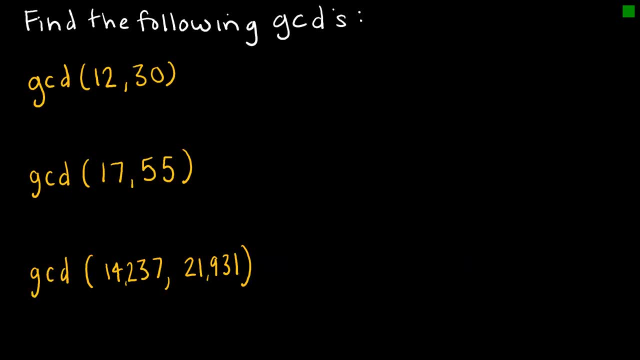 But obviously looking at primes is going to be sort of an easy way to go forward, since we're studying primes right now. So let's just do a little bit of practice. First one is 12 and 30. And again I can look at 12 and say: what's the prime? factorization? 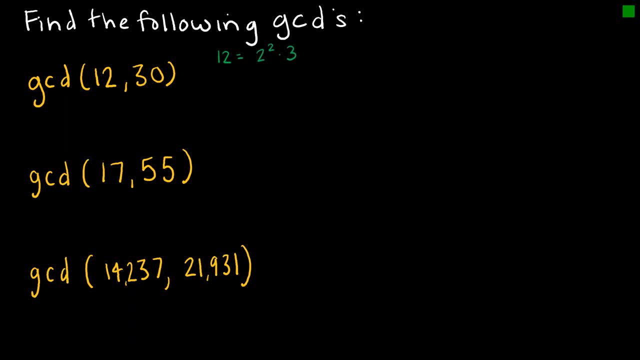 And 12 is 2 squared times. So 12 squared times 3, I can look at 30 and say 2 goes into it once. that gives me 15.. 15 is 3 times 5. And so my GCD would be the most number of times 2 occurs in common, which is just once. 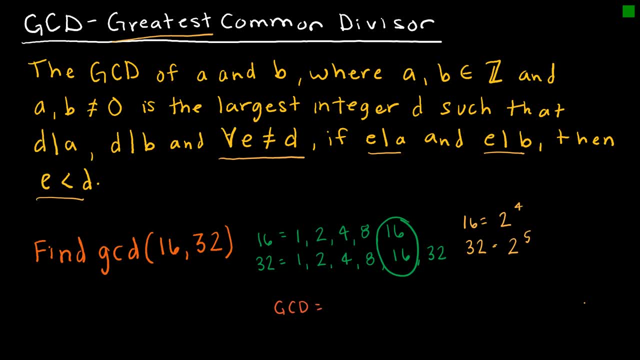 I'm looking at the most number of times that a prime occurs in common with one another. So here's 2 to the fourth, this is 2 to the fifth, So 2 to the fourth, and this is like 2 to the fourth times 2.. 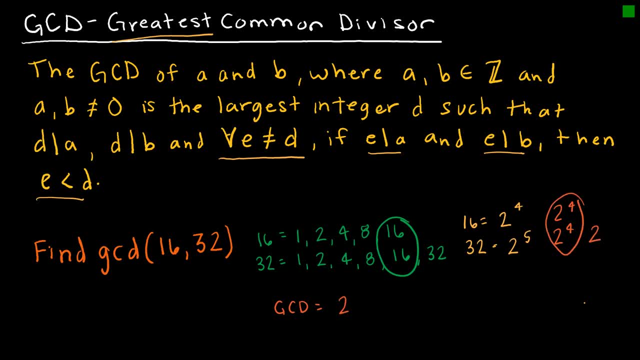 So 2 to the fourth is the greatest number of times that occurs in both, And so that is the greatest, And so that is the greatest common divisor, which is of course 16.. So the answer is 16, either way you look at it. 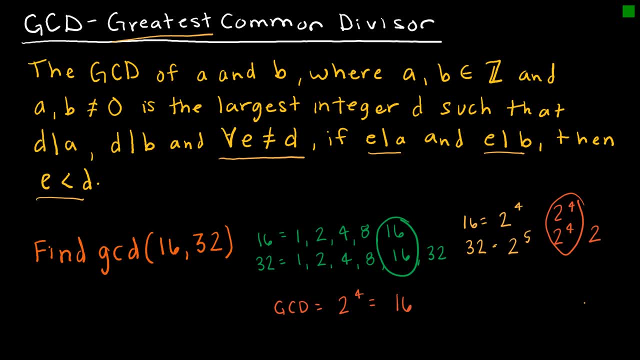 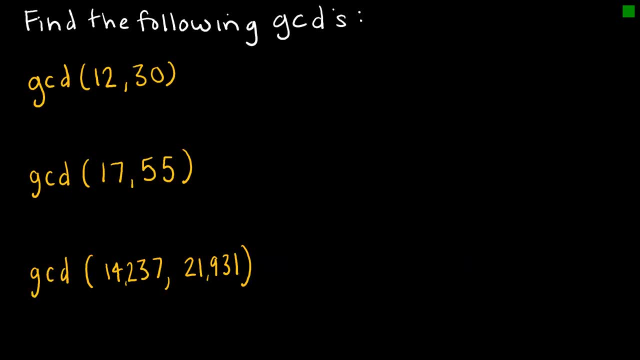 But obviously looking at primes is going to be sort of an easy way to go forward, since we're studying primes right now. So let's just do a little bit of practice. First one is 12 and 30. And again I can look at 12 and say: what's the prime? factorization? 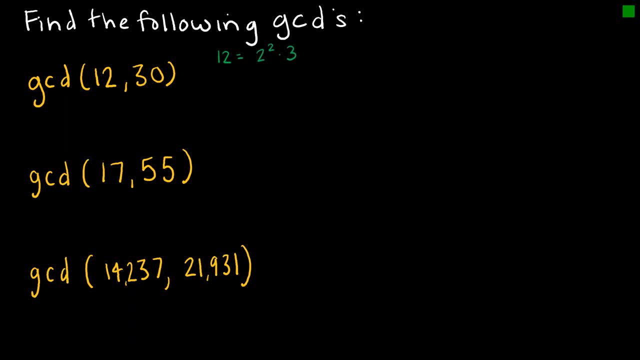 And 12 is 2 squared times. So 12 squared times 3, I can look at 30 and say 2 goes into it once. that gives me 15.. 15 is 3 times 5. And so my GCD would be the most number of times 2 occurs in common, which is just once. 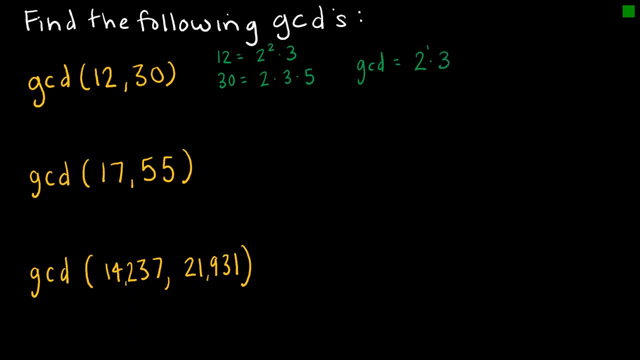 The most number of times 3 occurs in common, which is just once, And the number of times 5 occurs in common, which is it doesn't 5 to the 0. And so my greatest common divisor here would be 2 times 3, which is 1.. 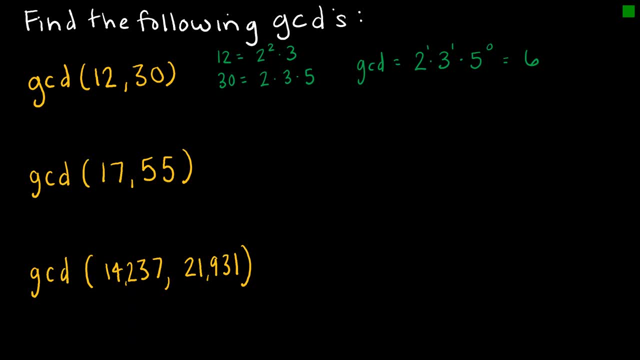 And so my greatest common divisor here would be 2 times 3,, which is 6.. Again, you might be able to just figure that out very easily by looking at 12 and 30, and that's great. I'm just showing you how we would do it, as we. as it pertains to primes. 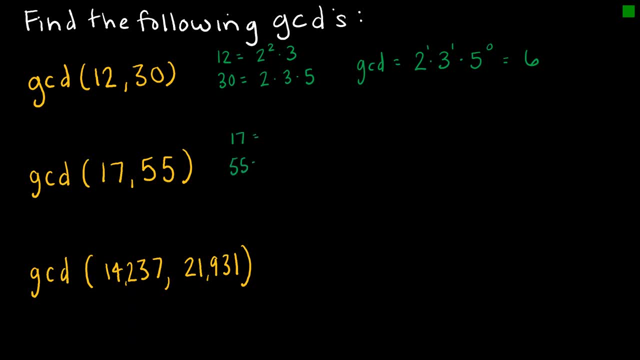 Same thing for 17 and 55,. 17 is a prime, So it's just 17,. 55, it's 5 times 11.. Those are both primes. So what is the greatest common divisor? It would just be 1.. 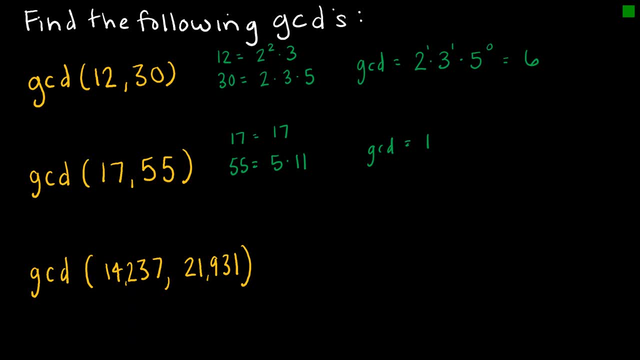 One is the largest number. that goes into both of those, And what I want to point out on this one is that this is considered relatively prime. So relatively prime means that they don't have any factors in common. So GCD of 1.. 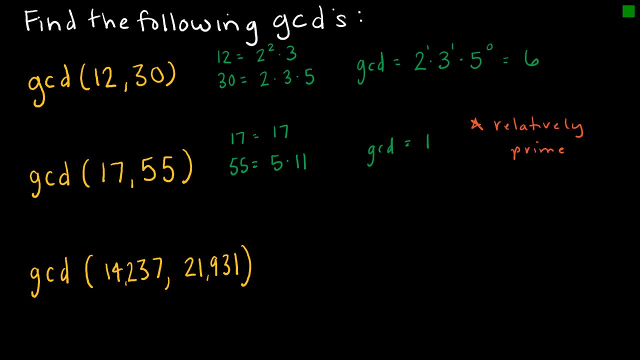 And then let's look at that last one. I don't know about you, but that just seems like something I don't want to do, I don't want to tackle, And so the reason I put it on here is to let you know there is a way to go about this. 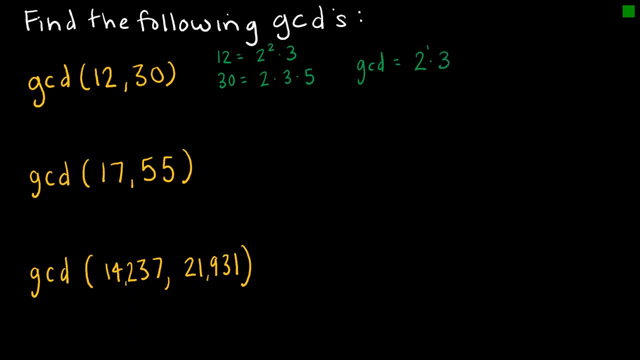 The most number of times 3 occurs in common, which is just once, And the number of times 5 occurs in common, which is it doesn't 5 to the 0. And so my greatest common divisor here would be 2 times 3, which is 1.. 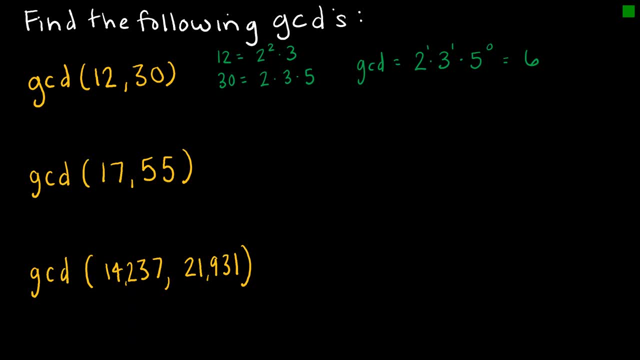 And so my greatest common divisor here would be 2 times 3,, which is 6.. Again, you might be able to just figure that out very easily by looking at 12 and 30, and that's great. I'm just showing you how we would do it, as we. as it pertains to primes. 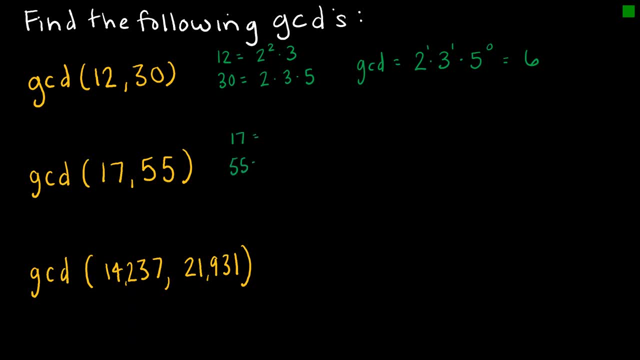 Same thing for 17 and 55,. 17 is a prime, So it's just 17,. 55, it's 5 times 11.. Those are both primes. So what is the greatest common divisor? It would just be 1.. 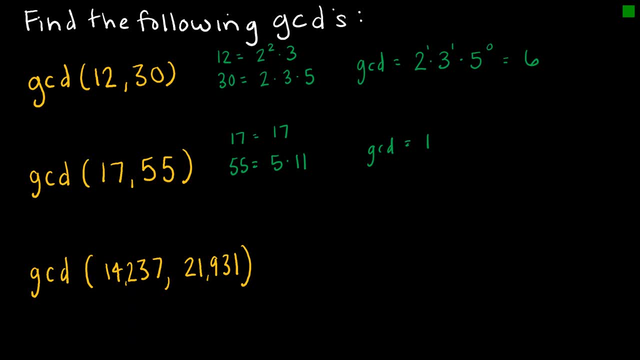 One is the largest number. that goes into both of those, And what I want to point out on this one is that this is considered relatively prime. So relatively prime means that they don't have any factors in common. So GCD of 1.. 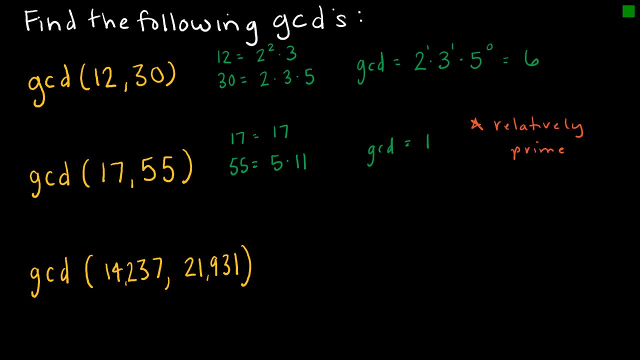 And then let's look at that last one. I don't know about you, but that just seems like something I don't want to do, I don't want to tackle, And so the reason I put it on here is to let you know there is a way to go about this. 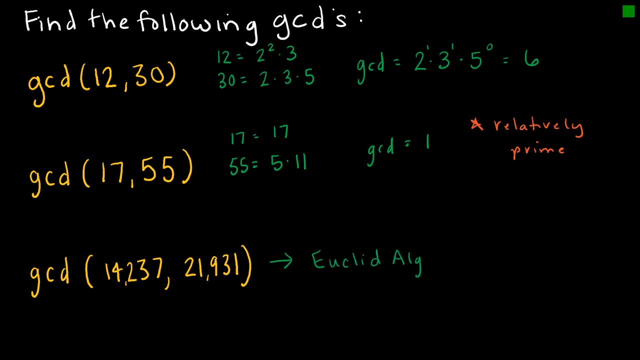 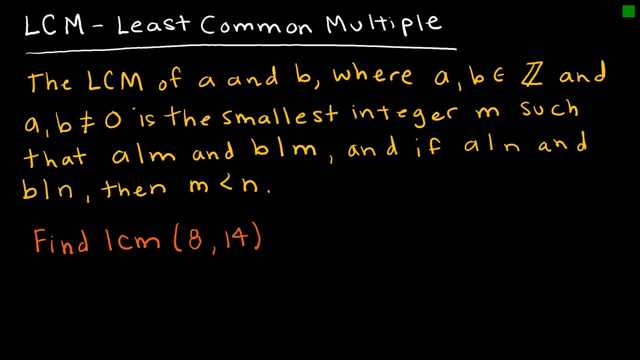 And it is Euclid's algorithm which we'll study in a little bit, But for now I'm not even going to try to find the greatest common divisor of those two values. So now let's look at the least common multiple, The least common multiple of A and B, where A and B are both integers and not equal to. 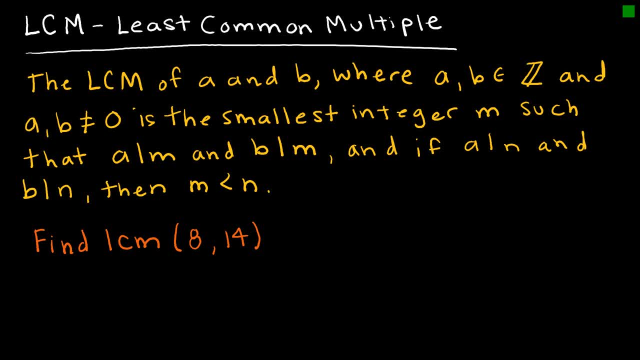 0. This is an integer that essentially divides, that they both divide. So A divides M and B divides M. And if there happens to be another integer that A divides and B divides, then M is the smallest of those, So it's the least common multiple. 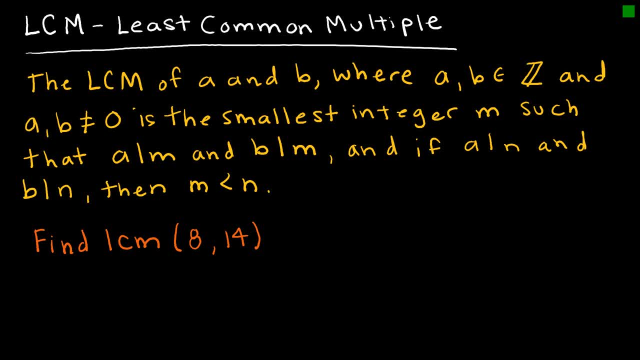 So, again for this one, instead of looking at numbers that multiply into 8, factors of 8,, I would be looking at 8 as 8.. 1. 16,, 24,, 32,, 40,, 48,, 56,, etc. 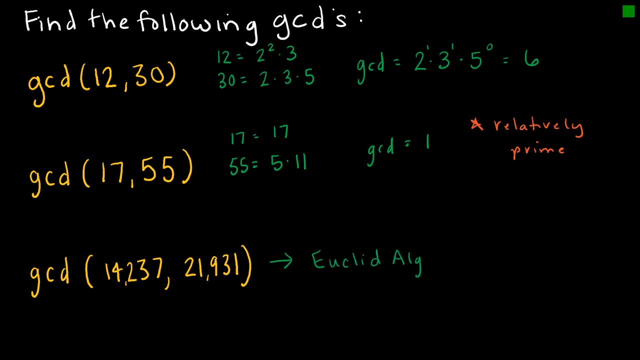 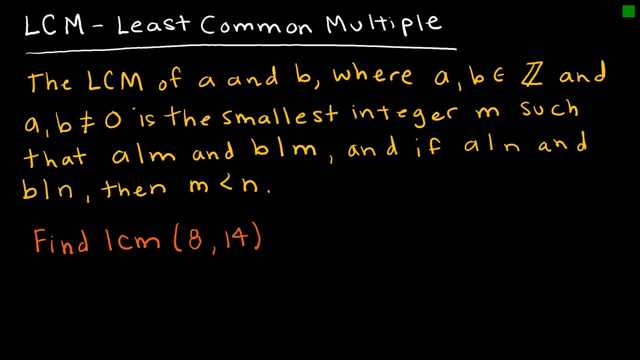 And it is Euclid's algorithm which we'll study in a little bit, But for now I'm not even going to try to find the greatest common divisor of those two values. So now let's look at the least common multiple, The least common multiple of A and B, where A and B are both integers and not equal to. 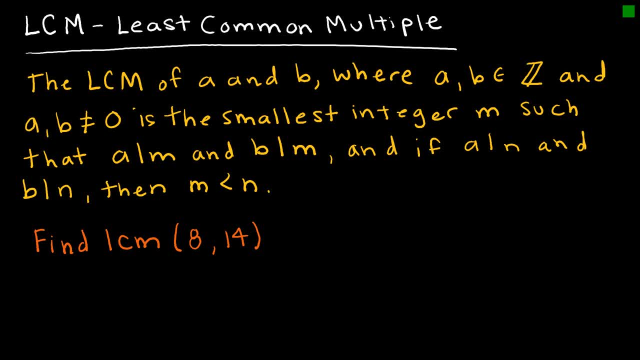 0. This is an integer that essentially divides, that they both divide. So A divides M and B divides M. And if there happens to be another integer that A divides and B divides, then M is the smallest of those, So it's the least common multiple. 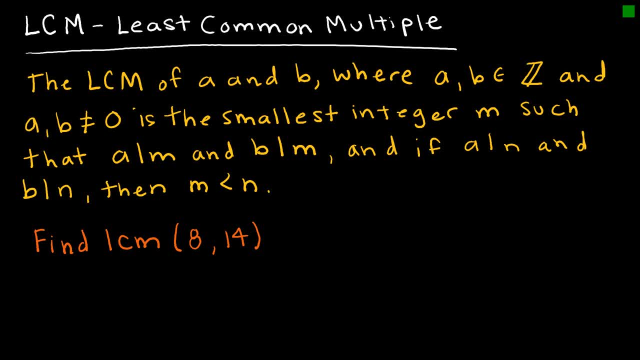 So, again for this one, instead of looking at numbers that multiply into 8, factors of 8,, I would be looking at 8 as 8.. 1. 16,, 24,, 32,, 40,, 48,, 56,, etc. 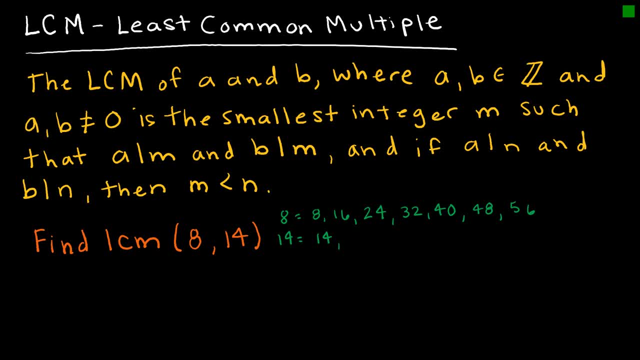 And 14 would be 14 times 1,, 14 times 2,, 14 times 3, and I can see I don't have one in common yet, And so this is where it's not so fun, Because then you just have to basically keep going. 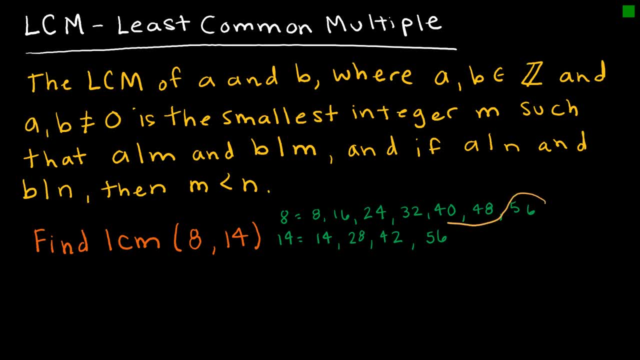 Until you find one, And so, in this case, I have found that 56 would be the least common multiple. So is there a way to use primes to do this, as we did when we looked at the greatest common divisor? Well, let's take a look at 8.. 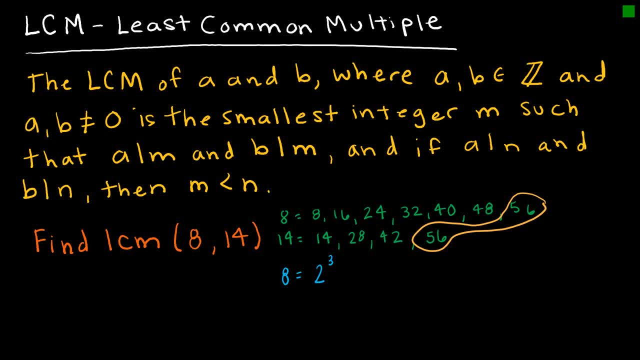 8 is 2 times 2 times 2.. And 14, prime factorization 2 times 7.. And so in our last example, when we were looking at the least common divisor, we found that the least common divisor is 2 times 2 times 3 times 4 times the least common divisor. 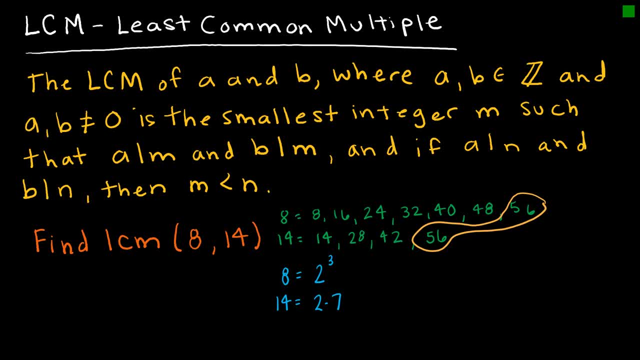 And so this is going to make it a little bit more complicated. So let's look at the least common divisor, And in our last example, when we were looking at the greatest common divisor, we said: how many do they have in common? And when we look at the least common multiple, we're looking at how many is the most number? 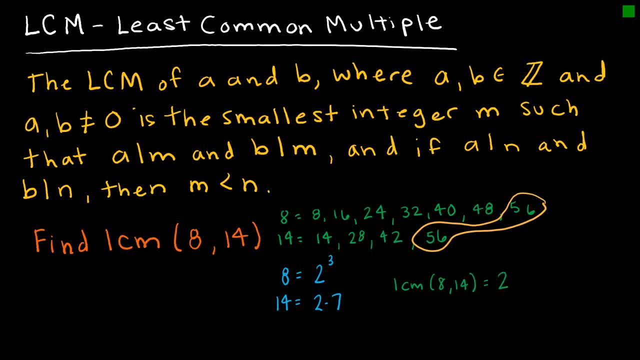 of times it occurs, So they have both have a 2.. What's the most number of times it occurs Three times. Only one of them has a 7, and it occurs one time. So the most number of times it occurs is once. 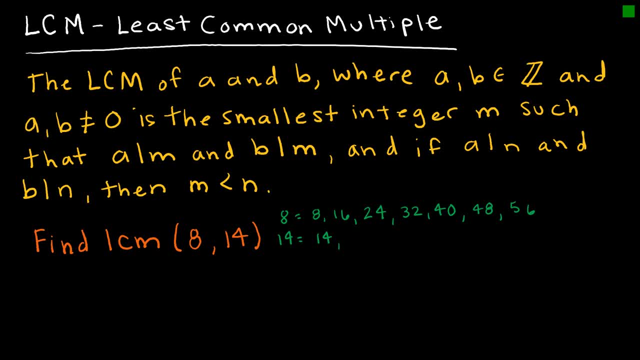 And 14 would be 14 times 1,, 14 times 2,, 14 times 3, and I can see I don't have one in common yet, And so this is where it's not so fun, Because then you just have to basically keep going. 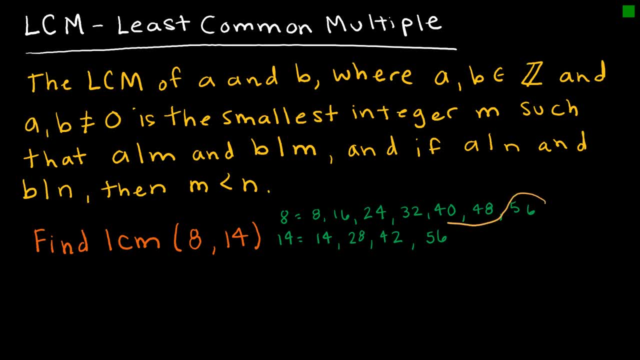 Until you find one, And so, in this case, I have found that 56 would be the least common multiple. So is there a way to use primes to do this, as we did when we looked at the greatest common divisor? Well, let's take a look at 8.. 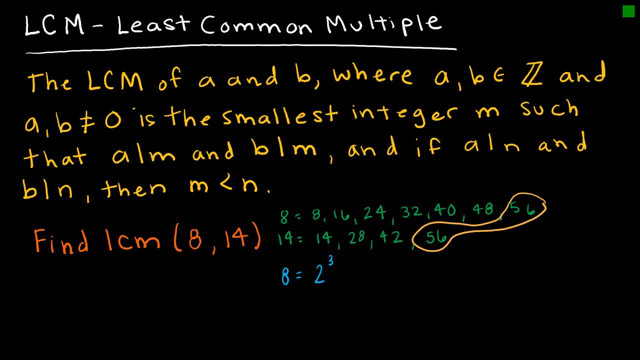 8 is 2 times 2 times 2.. And 14, prime factorization 2 times 7.. And so in our last example, when we were looking at the greatest common divisor, we found that 8 is 2 times 2 times 2.. 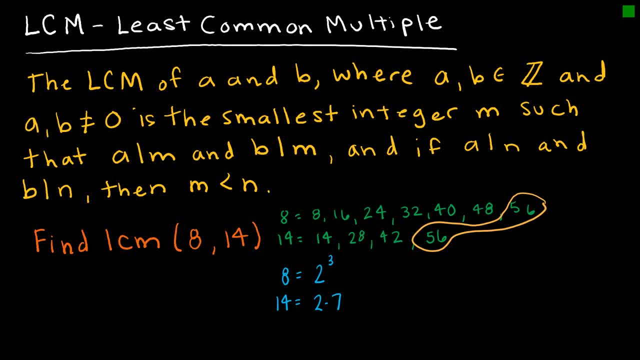 And so in our last example, when we were looking at the greatest common divisor, we said how many do they have in common? And when we look at the least common multiple, we're looking at how many is the most number of times it occurs? 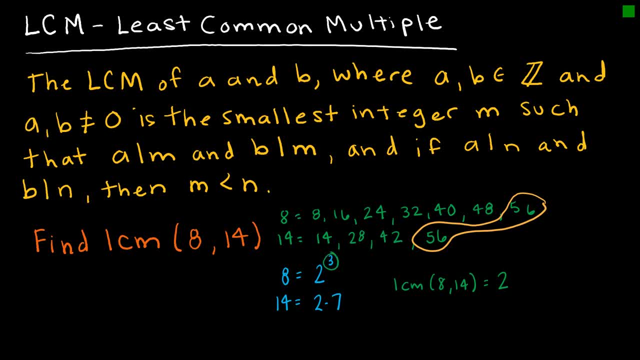 So they both have a 2,. what's the most number of times it occurs Three times. Only one of them has a 7, and it occurs one time. So the most number of times it occurs is once. So 7 to the first. 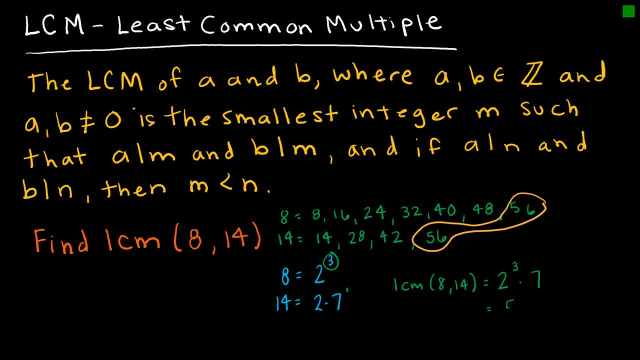 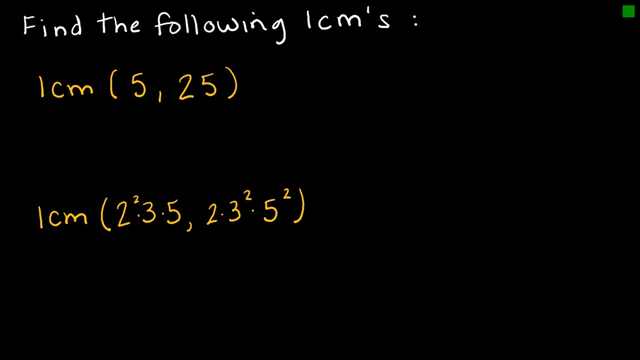 So then I'm just taking 2 to the third times 7, which is 56. So again, this is a strategy for us to use, especially if we already have it written as a prime factorization. So again, just a couple of practice, pretty straightforward. 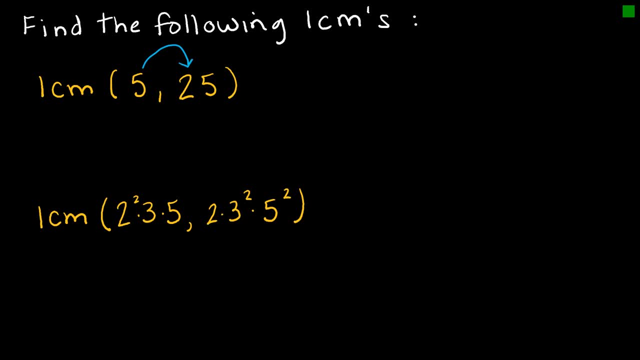 One thing that you can do right away- which is why I included this example- is you can say: does 5 go into 25?? Because if it does, there's your LCM right there, So you don't have to do any additional work because you know that that's the smallest. 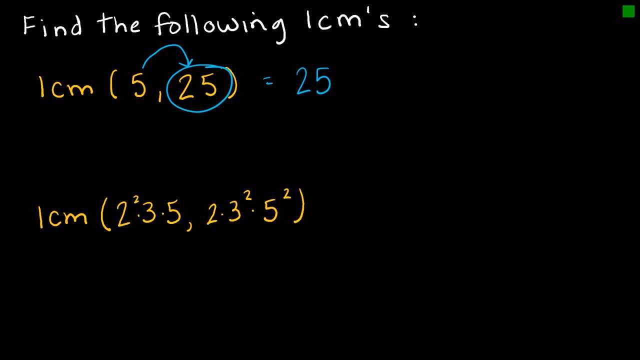 number that they're both going to divide into. And the second example I've included because it's already in my prime factorization And so again I'm just going to use that strategy where I say the most number of times 2 occurs. 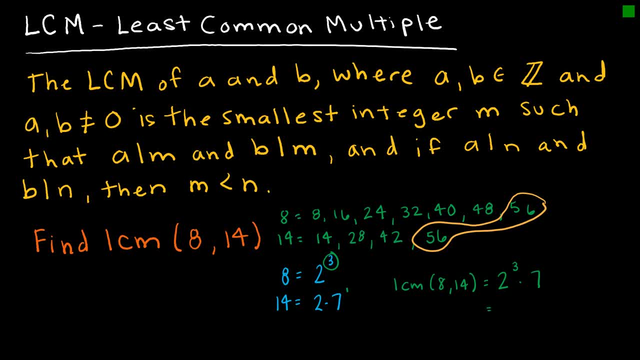 So 7 to the first. So then I'm just taking 2 to the third 4 times. So that's how I'm going to do this: 2 to the third times 7, which is 56. So again, this is a strategy for us to use, especially if we 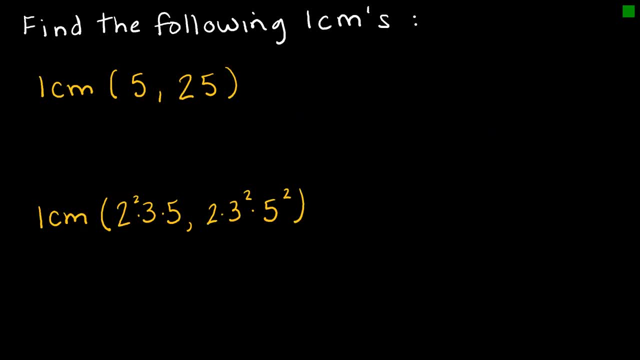 already have it written as a prime factorization. So again, just a couple of practice. pretty straightforward. One thing that you can do right away- which is why I included this example- is you can say: does 5 go into 25? because if it does, there's your LCM right there. you don't have to. 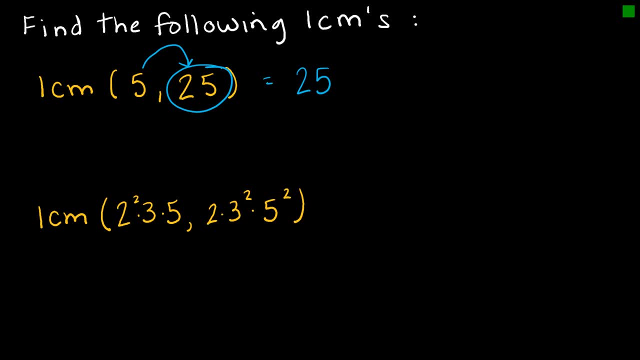 do any additional work because you know that that's the smallest number that they're both going to divide into. And the second example I've included because it's already in my prime factorization and so again, I'm just going to use that strategy where I say the most number of times. 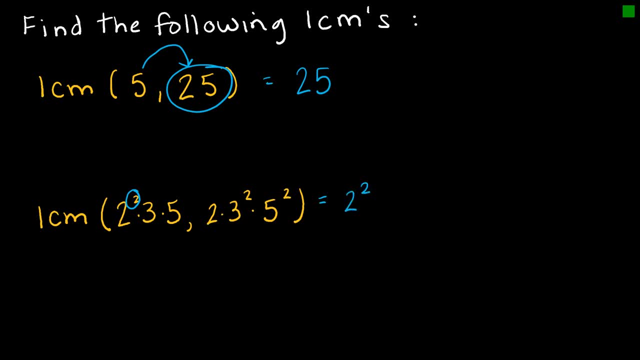 2 occurs is twice, the most number of times 3 occurs is twice and the most number of times 5 occurs is twice. So if I multiply all of that out then I get 900, and 900 is my least common multiple and I saved myself a bunch of time. 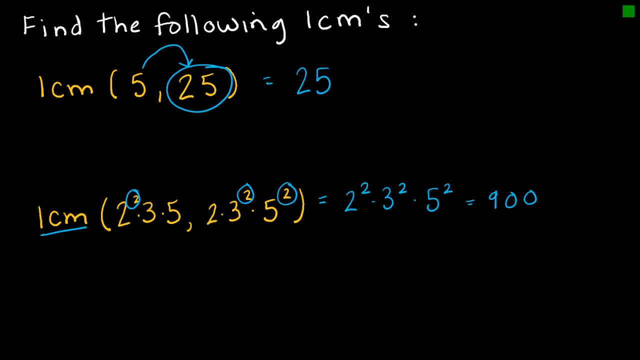 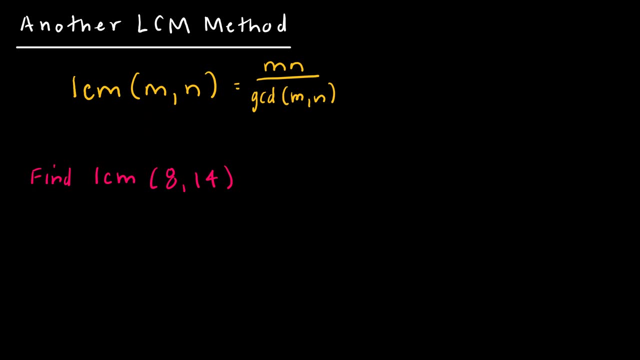 from having to write out all of the multiples of each number. There is one more method for finding the least common multiple, and it involves the greatest common divisor. So, as we can see, to find the least common multiple of two integers, we could multiply those integers and divide it. 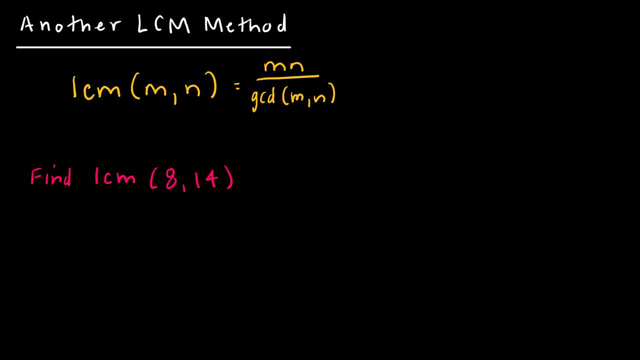 divide that product by the least common divisor. So if I write out all of the multiples of each of the integers, we could multiply the greatest common divisor of the integers. So previously we found the least common multiple of 8 and 14 and we said that that solution was 56. So let's see if we 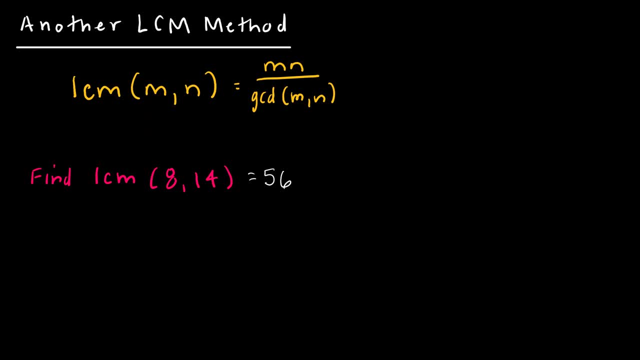 get 56 again using our new formula. So in this case we would say least common multiple of 8 and 14 would be 8 times 14 divided by, and this would be the greatest common divisor. So again we're saying what is the largest. 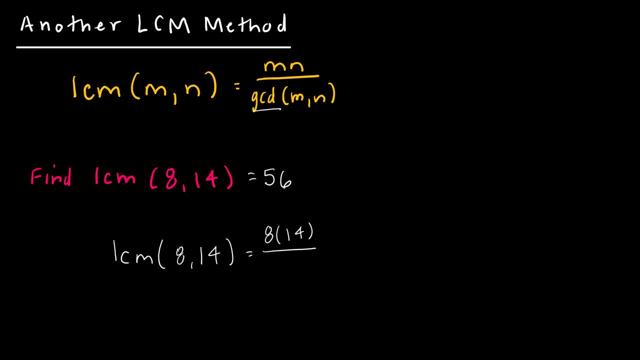 number that goes into 8 and 14, and you can do that in whichever method that you'd like. Again, if I said 8 was 2 to the 3rd and 14 is 2 times 7, this is where I'm looking for the most that they have.